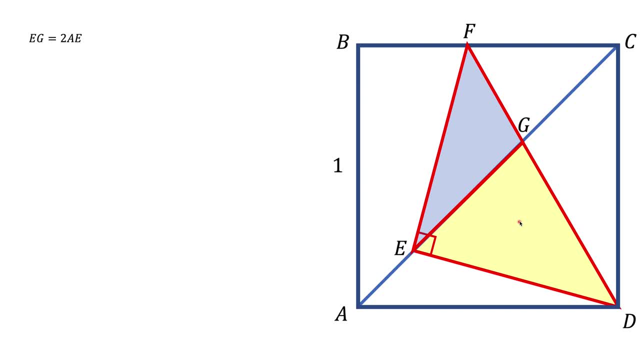 us the right triangle. The next thing we are going to do, we are going to connect point A and F And we are going to get four triangles here: Our original blue and yellow, but we also get gray and pink triangles Together. they are going to give us one big triangle. AFD. 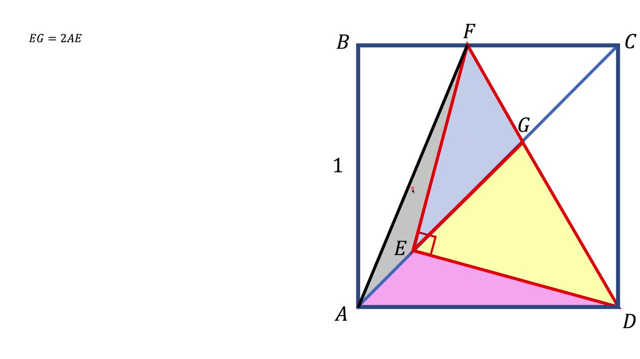 So first of all, let's look at the blue triangle and the gray triangle. Triangles are the same triangles that lay above the diagonal AC. Let's compare these areas. Well, we know that the area of a triangle is half high times the base. So let's drop an altitude: FH. This is an altitude or height of both blue and 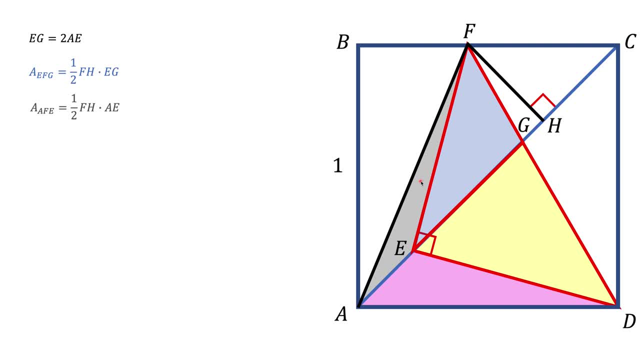 gray triangles And the areas of those two triangles will be half that altitude FH times. in the case of the Blue Triangle, a bit of an AC. Let's add aшт to the A, so we have an altitude FH and a Н. The area of the two triangles is going to be the same. 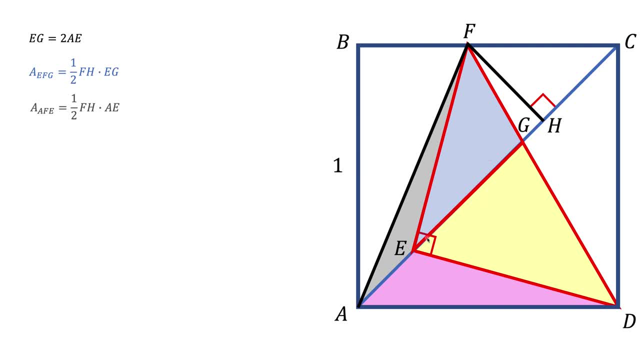 too, and we are going to divide this triangle into two homem makeup spiders. The Cartier Triangle is This side EG and in the case of gray triangle is the side AE. And since AE is a half of EG, what we find from here is that the area of the gray triangle is a half of the area of the blue triangle. 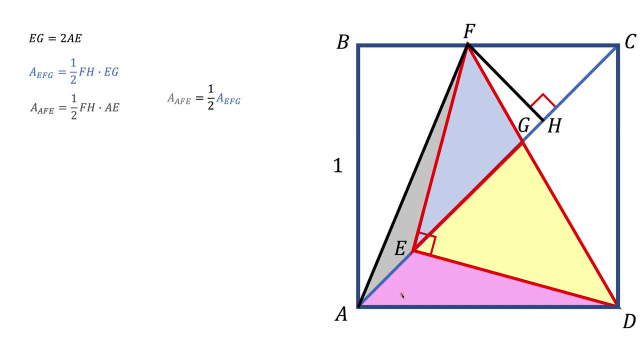 In a similar manner, we can show that the area of the pink triangle is a half of the area of the yellow triangle. The next thing to notice is that the triangle AFD, the big triangle, consists of four triangles: gray, blue, yellow and pink. 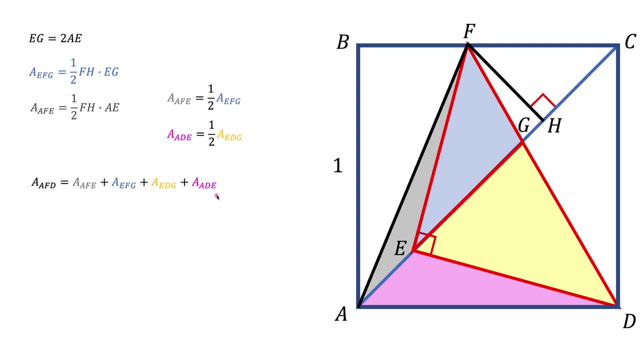 And that's what we have here And now. what we're going to do, we're going to use these two formulas to calculate the area of the gray triangle and the pink triangle And, if we do, we're going to have the area of the big triangle, AFD. 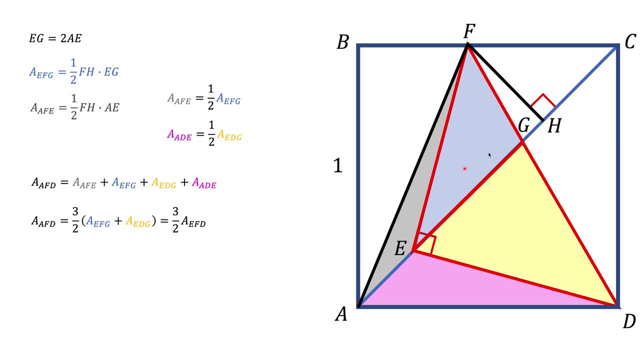 AFD is three halves of the area of the blue triangle and the area of the yellow triangle, But those two areas together give us the area of the triangle we're interested in And that is triangle EFD, And that's what we have here. 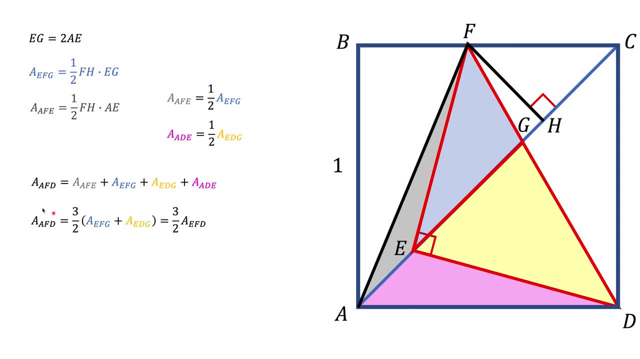 So now all we need to do is to find the area of the big triangle AFD. In this case, we can quickly find the area of the triangle EFD, But the area of the big triangle AFD- AFD is actually half of the area of this square. 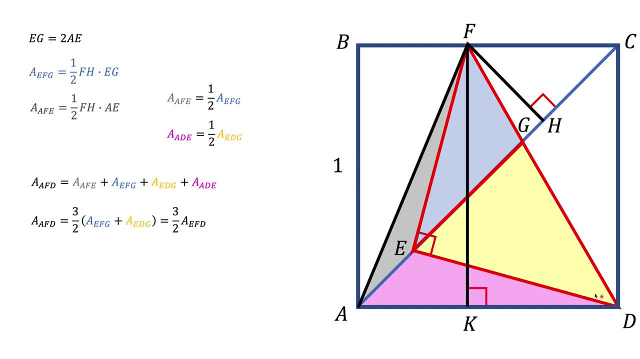 Why is that? Well, first of all, let's just drop an altitude in the big triangle, altitude FK, And now what we find is that the area of the big triangle AFD is half the altitude FK times the base AD. But FK equals to AB and equals to AD, and both of them equals to 1.. 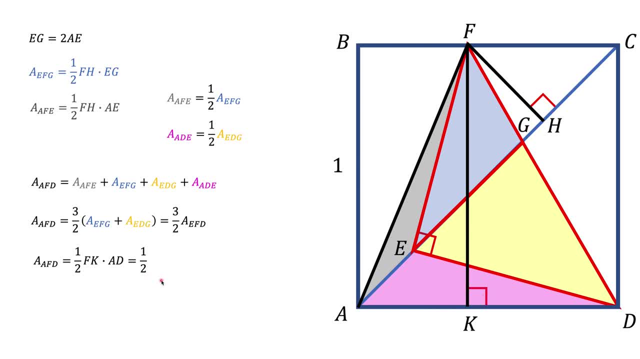 And therefore the area of this triangle is going to be half. Now, if you plug this half into previous equation, we can quickly see that the area of the triangle EFD is one. third Interesting observation is that originally we were given that the triangle EFD is a right triangle. 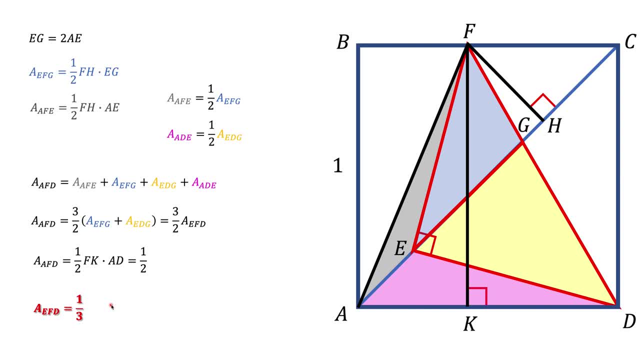 But if you look at the solution to this problem, we actually never use the fact. In fact, it doesn't. It doesn't really matter that this triangle is a right triangle or not a right triangle. So because of that, I really don't know why the author of this problem insisted on having triangle EFD as a right triangle.